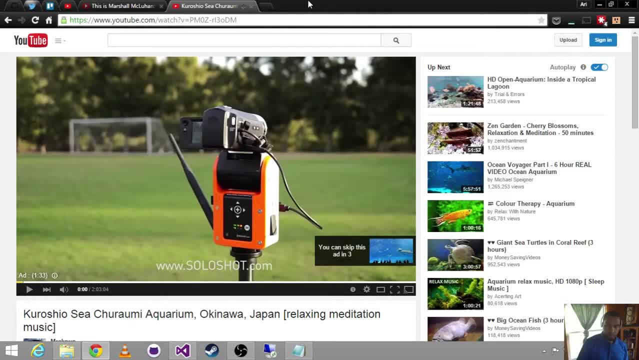 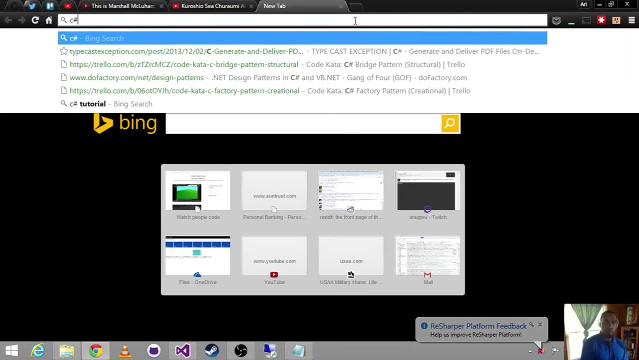 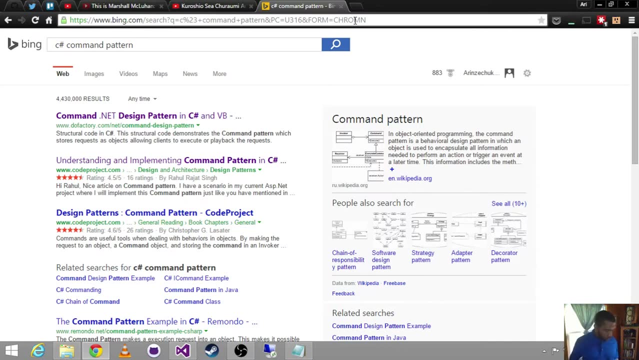 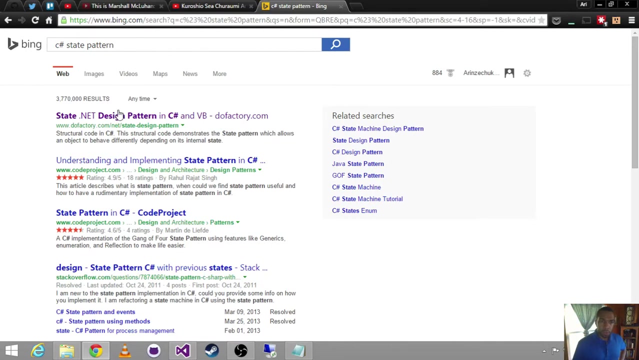 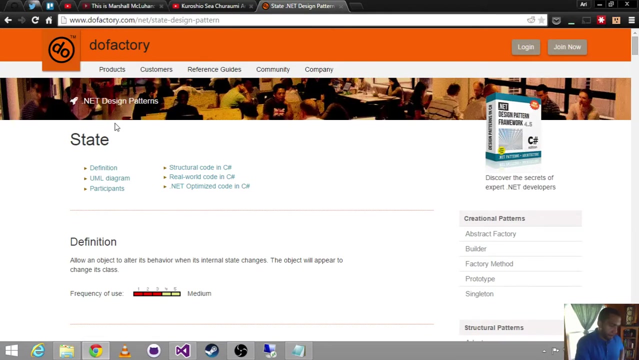 All right, So it is very hot in my little office. Summer has come to Virginia, So I was gone last week, Back today, to do the state pattern and also get back in the swing of things. So let's look up what the state pattern actually is. 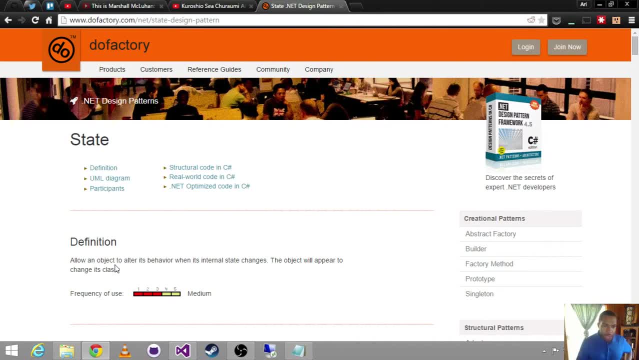 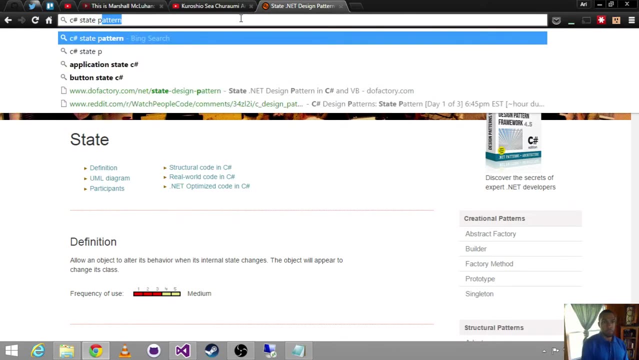 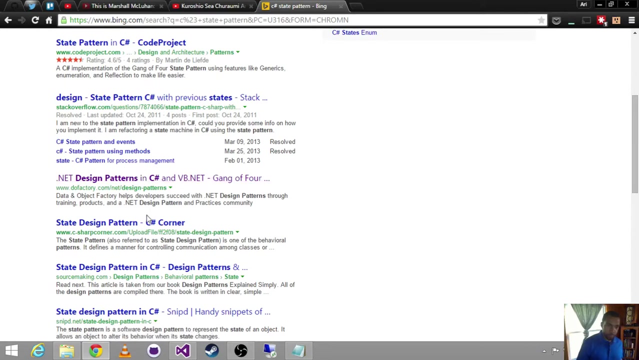 All right. So the state pattern allows an object to alter its behavior. when its internal state changes, The object will appear to change its class. That's fair. Let's see if we can get another one, just to see if there's any variance out there. 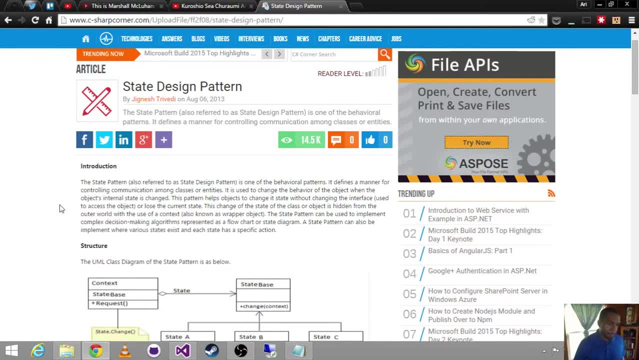 How about this? All right, The state pattern, also referred to as the state design pattern, is one of the behavioral patterns. It defines a manner for controlling communication among classes or entities. It is used to change the behavior of the object when the object's internal state is changed. 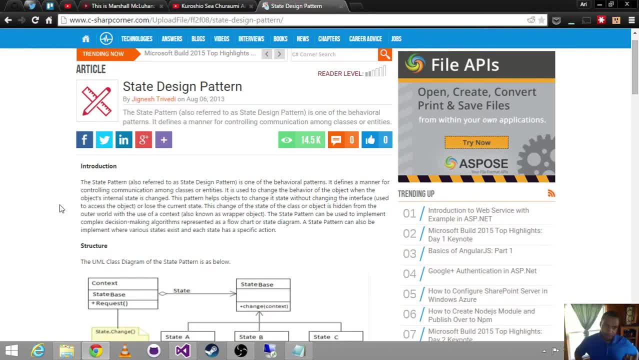 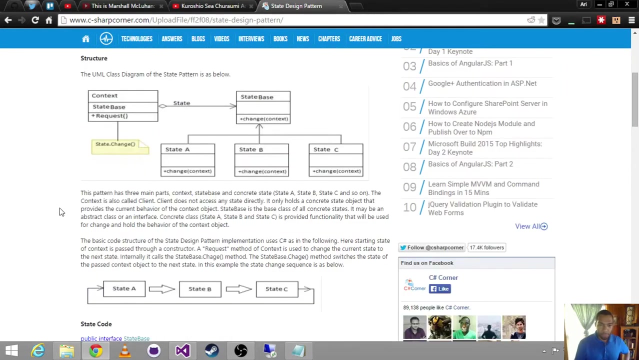 This pattern helps to change its state without changing the interface. Blah, blah, blah. This change of the state of the class or object is hidden from the outer world with the use of a context also known as a wrapper object. Okay, That's a lot of chatter. 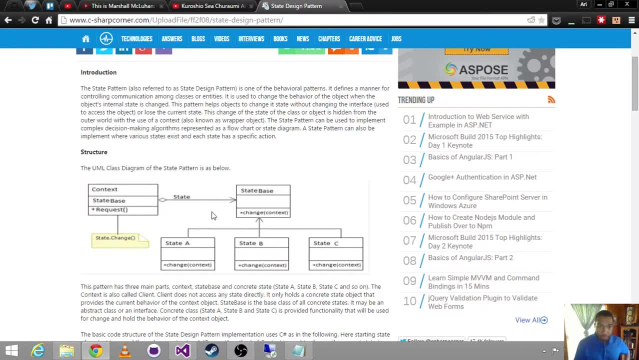 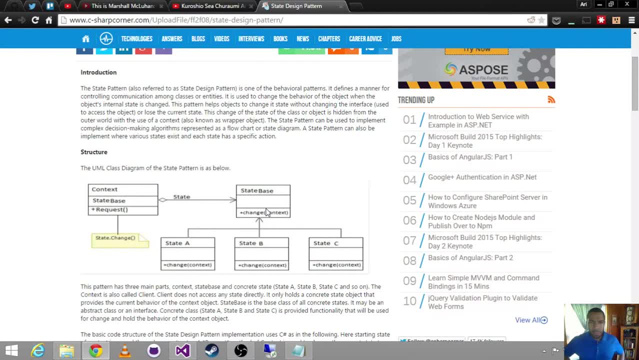 It's that there's often also a field or a property backing it. This is fine, And as a behavioral pattern, you'll start to see that they're all very, very similar, And so this is actually very similar to the strategy pattern. 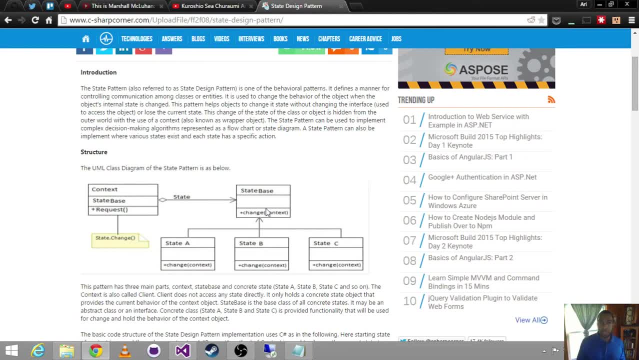 in the sense that we want to be able to change the strategy at will which affects the behavior, which affects the object representation. This is doing very much the same thing. So why is it different? Well, in a lot of the Deaf and Hard of Hearing classes, 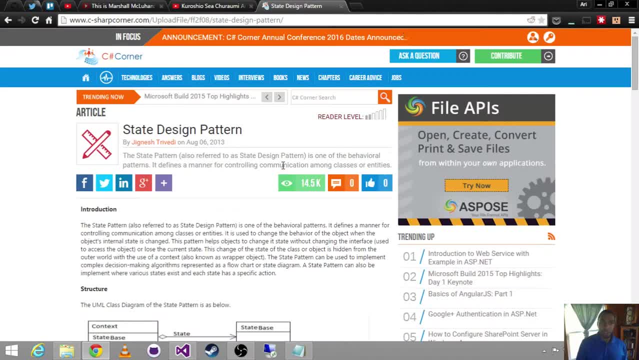 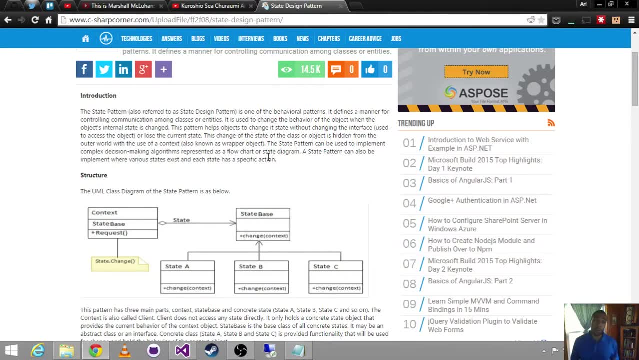 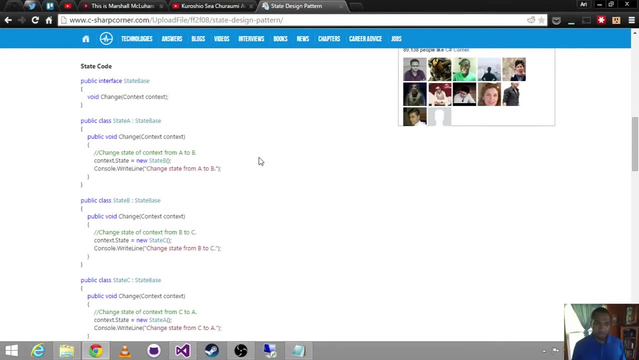 anything that you read, it's not different, And that's one of the issues with, I guess, design patterns is: there's a lot of overlap in their use, a lot of interpretation. people run off the reservation when something doesn't suit them. That's just the way it all kind. 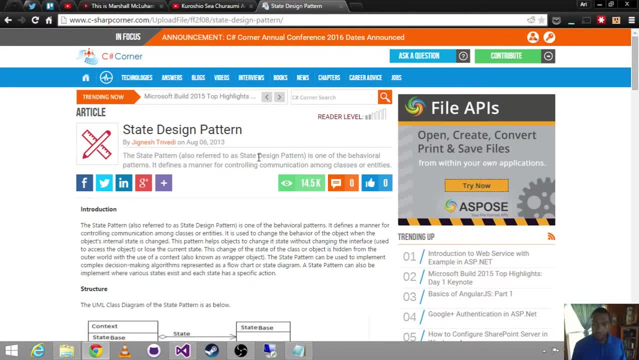 of rolls downhill, I guess. So what we're going to do is we're going to create the state design pattern via Kata, so that we can see what that looks like in code, and also try to make points where we want to use this approach over the strategy. 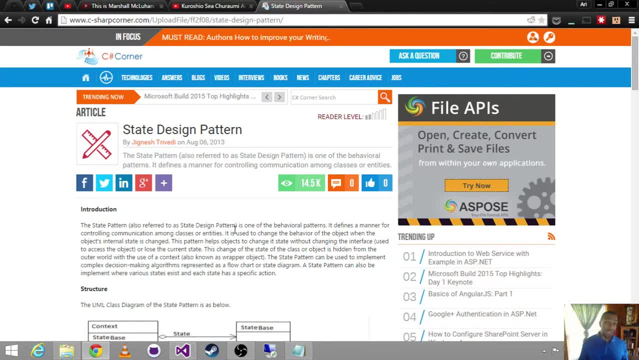 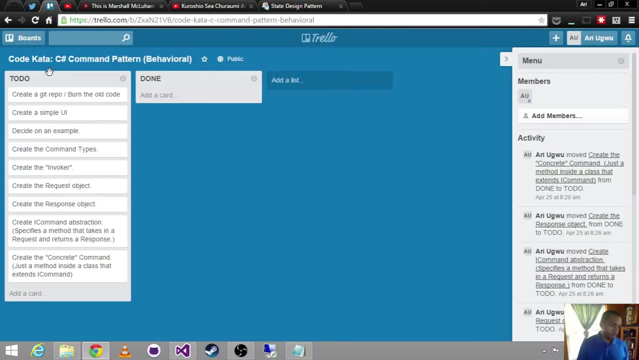 pattern because they are so similar, And if we can't find one, it just comes down to semantic sugar and use whichever one you think is best, But I think we will. So let's go over to Trello, And Kata is actually pretty simple. Oops, If I was on the right. 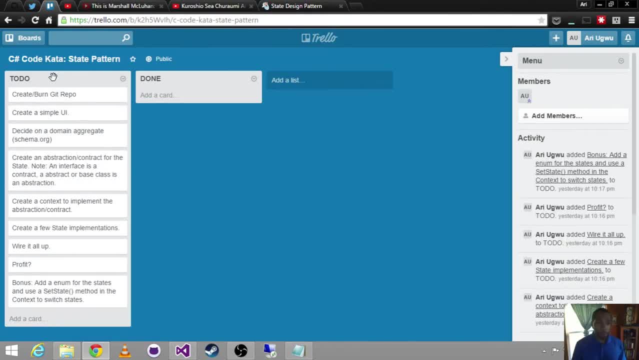 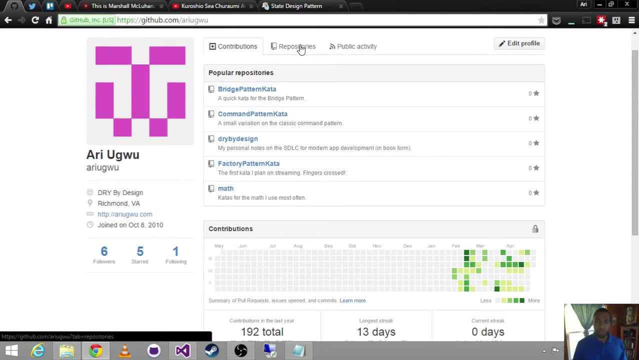 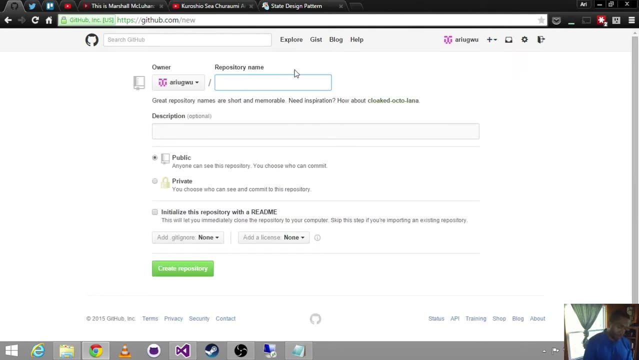 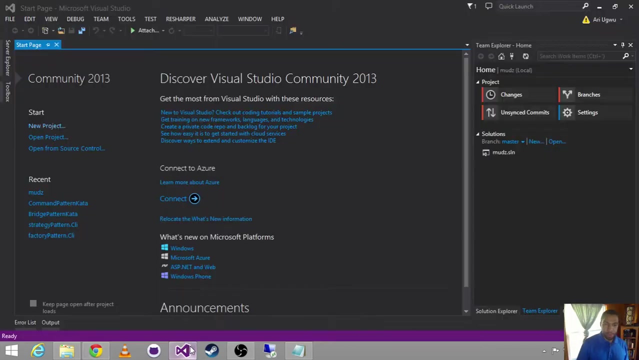 one, All right. So pretty simple as they all are, Let's go ahead and get started with our Git repo. So create a new repository. It's called state pattern, Kata. Okay, Go ahead and create that repository. Grab our link. 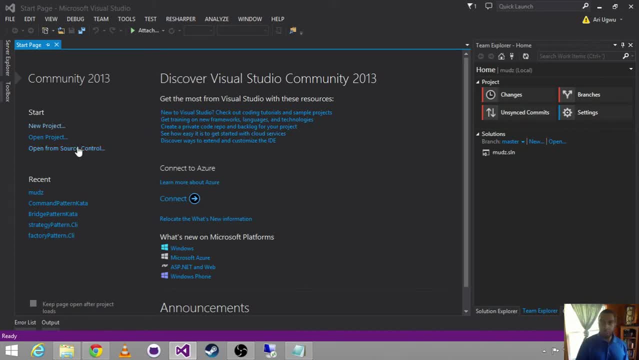 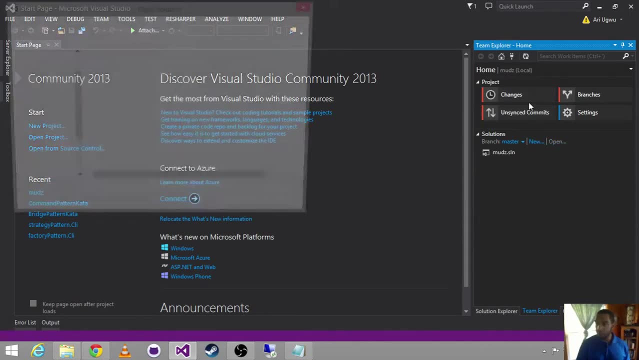 And here we go. We've created a new repository, So we're going to go ahead and create a new repository. Okay, We're going to come into Virtual Studio, Community 2013.. Go to Source Control And up there, Did you go home first? 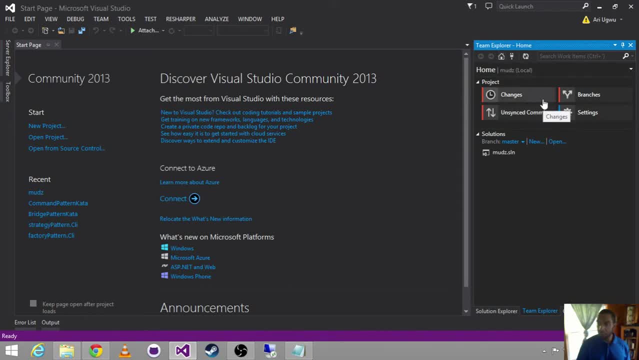 Oops, yes, Oops, all right. Connected Team Projects. So under Connected Team Projects we want to do a clone. I'm just going to paste in that URL And where it's going is fine, All right, it says to be cloned. 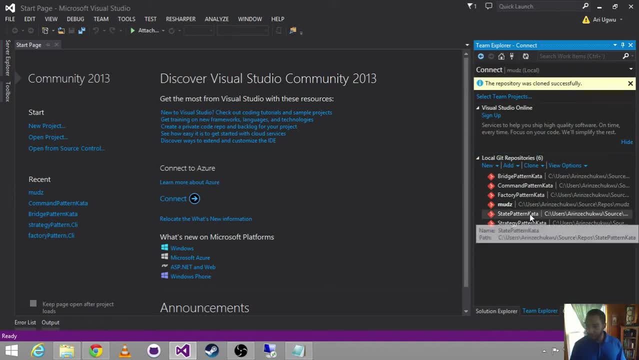 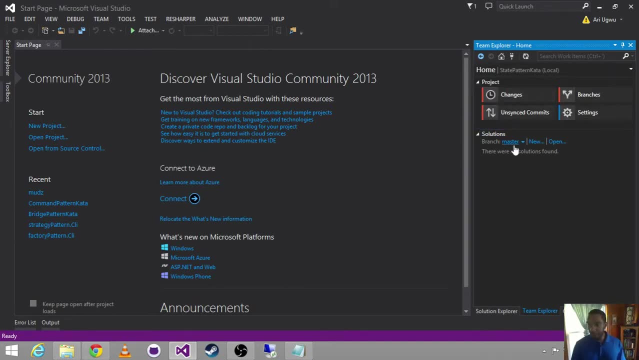 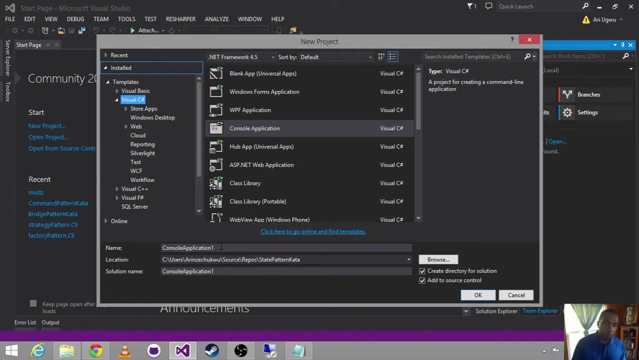 because there isn't a whole lot there And let's double click on that. So now that we're in the state pattern local repository And go under the master branch for solutions, Don't have any, Let's go ahead and make a new one. 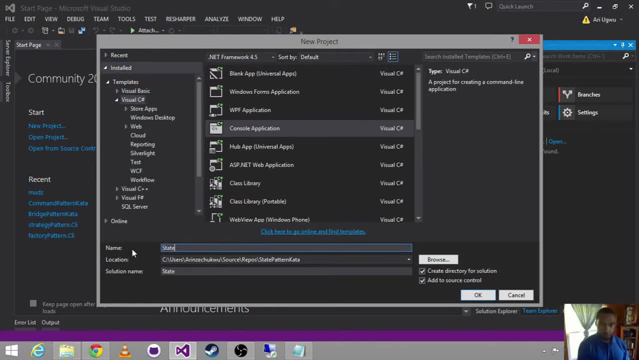 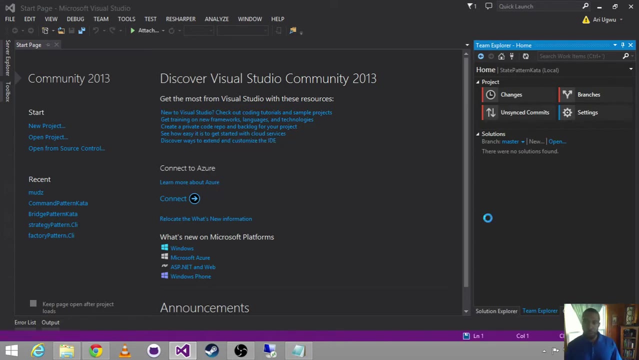 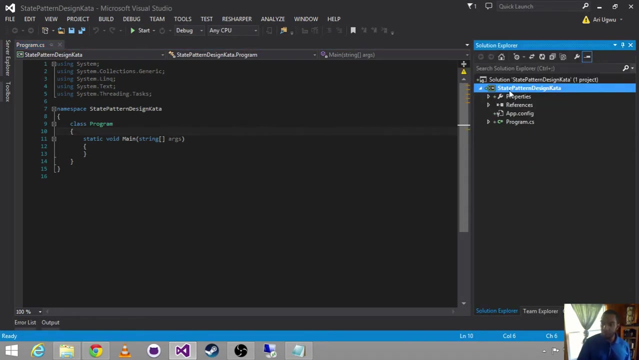 We're going to do the console application State pattern Design cover. We're ahead of C. it looks good, Okay, so let's go ahead and commit that. So under my solution explorer I'll right click and go to Commit. And I'll just say again: right click commit. I'll just say right click, commit. And I'll just say again: right click, commit. So I did my solution explorer. I'll right click and go to commit And I'll just say again: right click, commit. 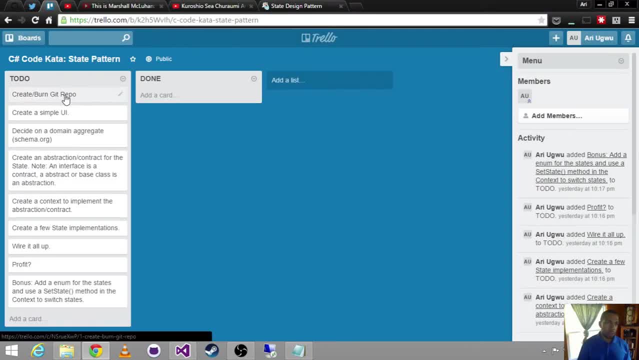 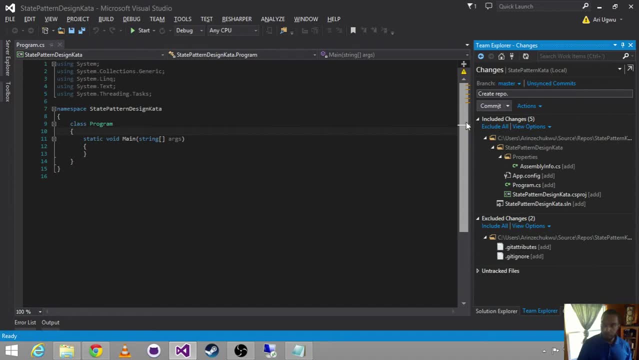 And I'm going to choose the next little right from our kata. I'll say: create or burn git repo. So I'm just going to do create repo, Commit and sync, Oh here. okay, we'll hang on Interesting. I think I heard remote ref to merge was not fetched. 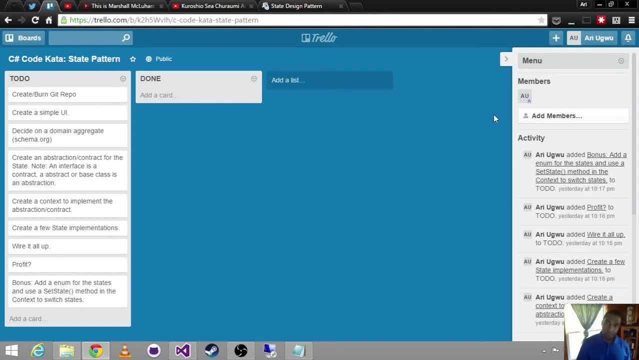 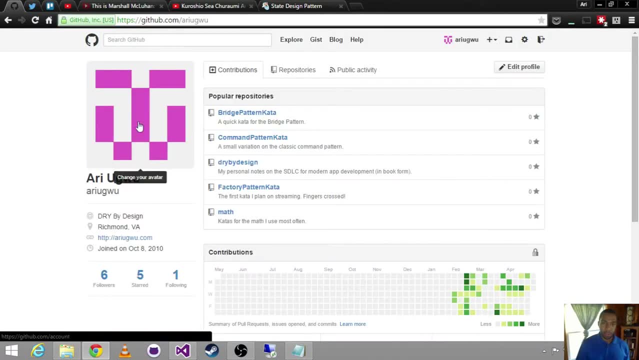 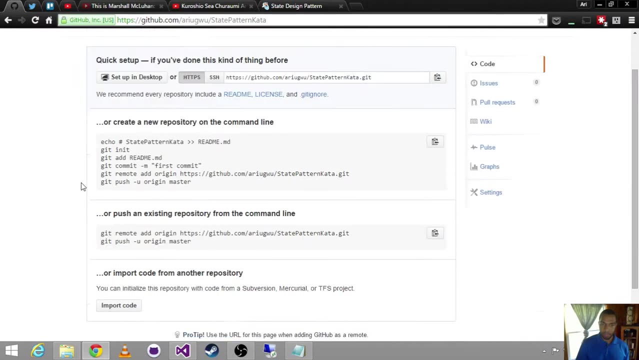 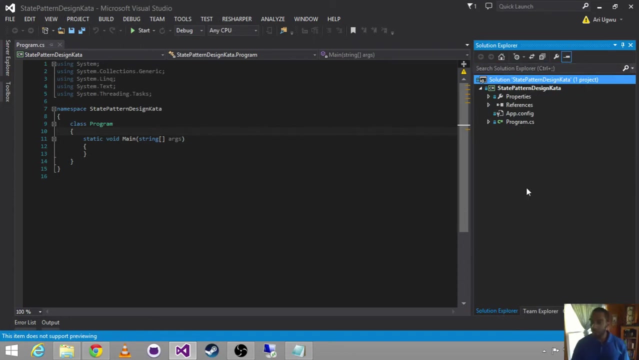 Zach says: hi, programmer. Hello back to you, Zach, fellow programmer. GitHub is being a little finicky tonight. Okay, so we might leave this. We're still going to commit to our local repo every time, And then you'll be able to follow along tonight probably. 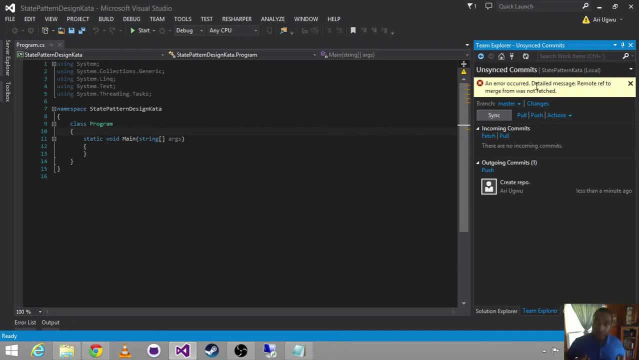 since GitHub is giving me some weird pushback, But once I do commit they should all come in order so you'll be able to follow along if you want to come back, Because I've never seen that and I'm not super sure why it cares. 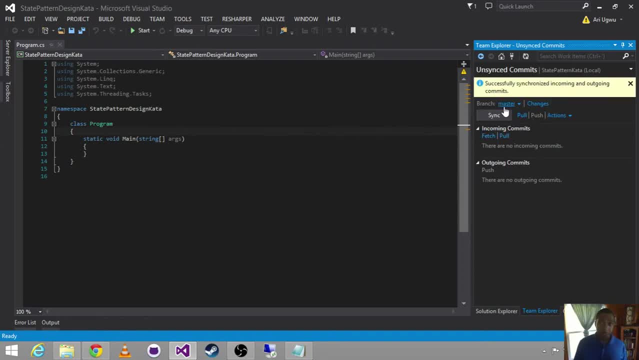 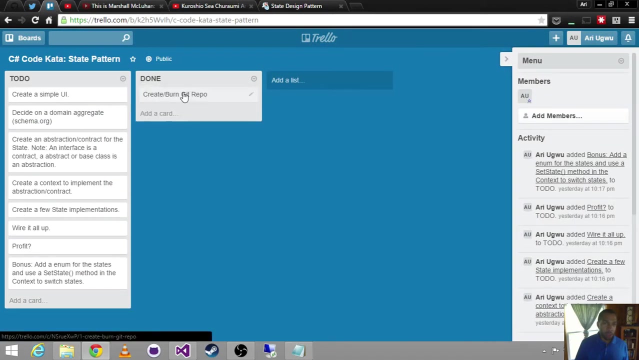 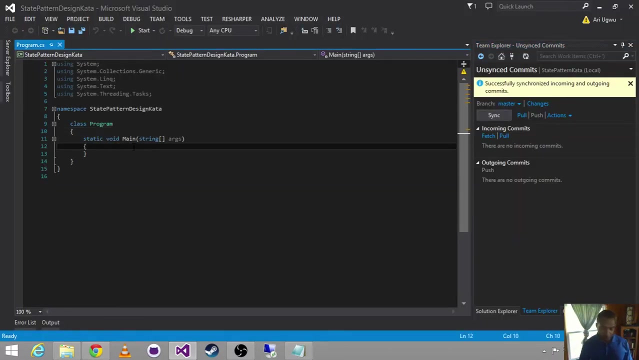 Okay, So maybe it's a network error. Okay, so let's come back over here and we created the git repo. Next up is to create a simple UI. Again. these first two steps, same ones for every cata. We're going to do a consolewriteline. 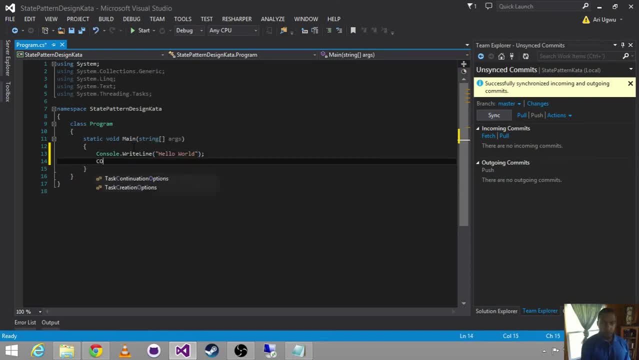 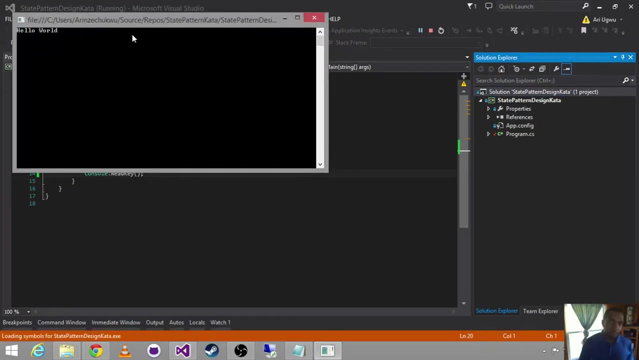 Hello world Console. Let's do a read key. Let's go ahead and just play this. Run it All right, so hello world. So this establishes that we've got a you know kind of a, a last known good state. 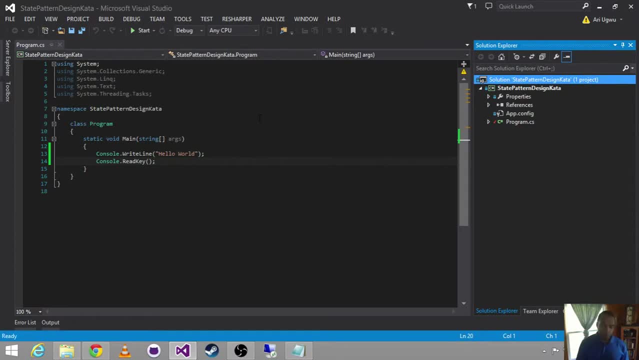 So, before doing anything but the simplest of tasks, we know that our environment is up and running, we know we're good to go, Which, as you just saw with the error from GitHub, is not something you can assume, even with some pretty robust, reliable services. 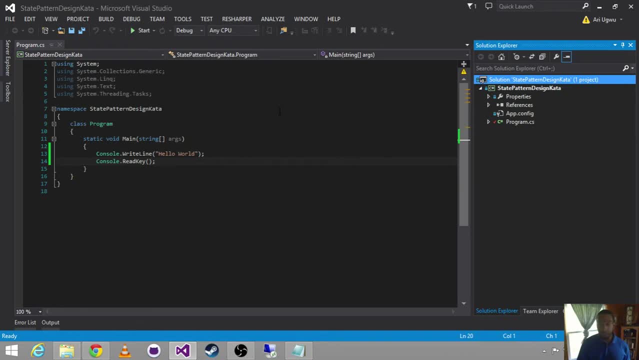 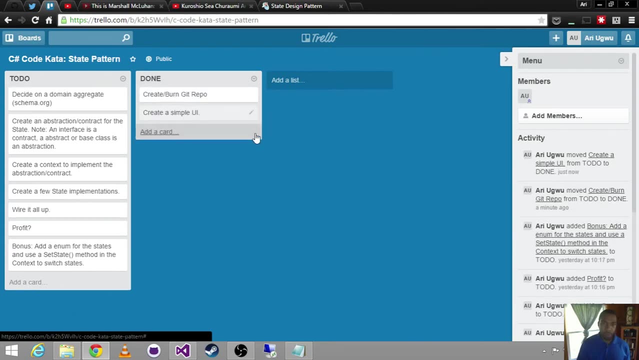 So this time it looks like it was on them, or maybe my network connection, but you'd just be surprised how much time can be lost. Okay, All right, So create a simple UI And done. All right, So the site of a domain aggregate. 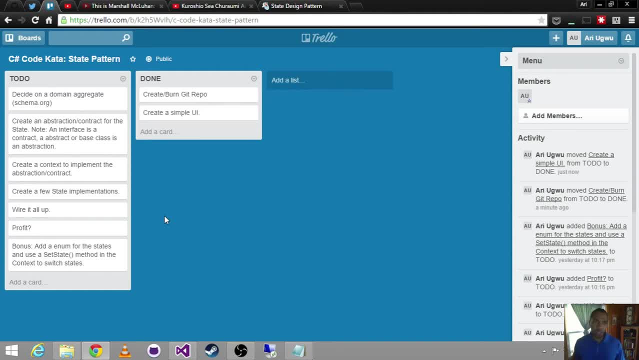 So if you've watched other videos or you're just joining, it's good to remember that we're doing a domain-driven design. That's my preference. It's going to affect the way that I structure the folders and a lot of the code. 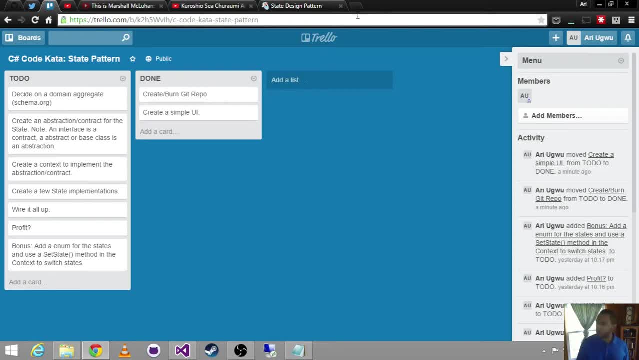 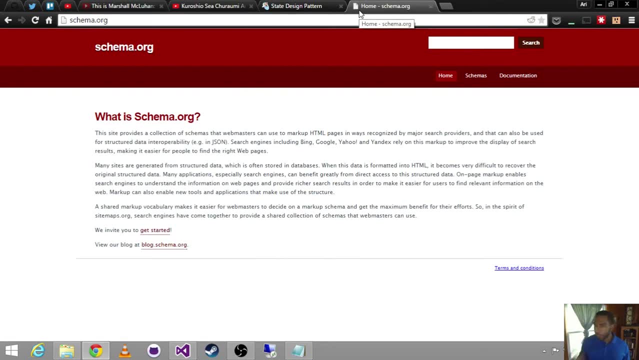 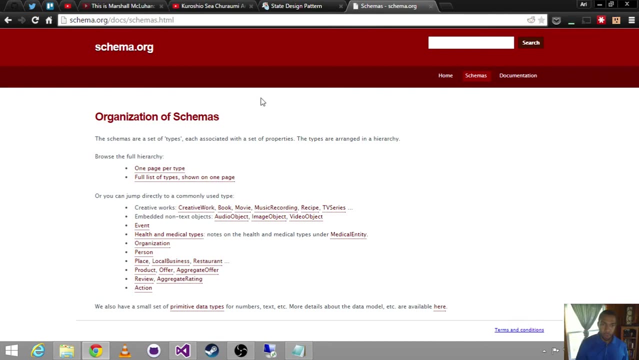 But I recently came across schemaorg. So if you're doing catas or you just want to have some kind of code, you can do that. I've got some ideas for how to model things. I found schemaorg to be pretty nice. 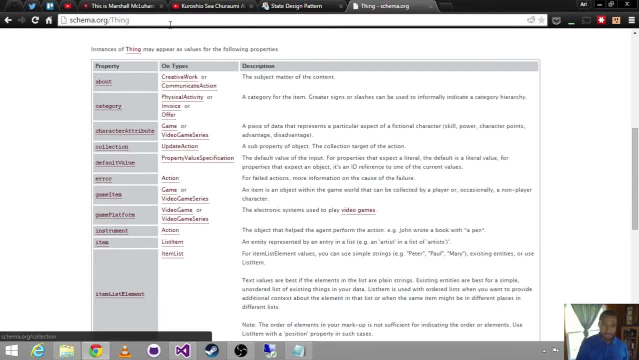 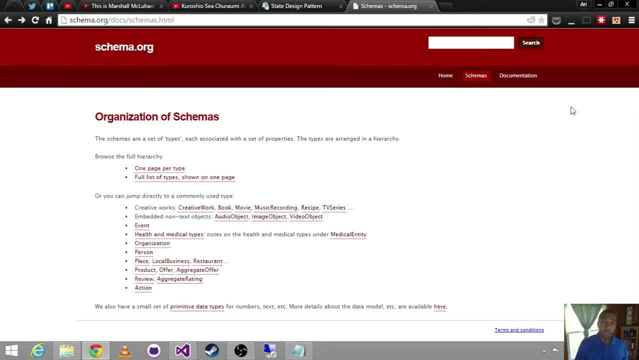 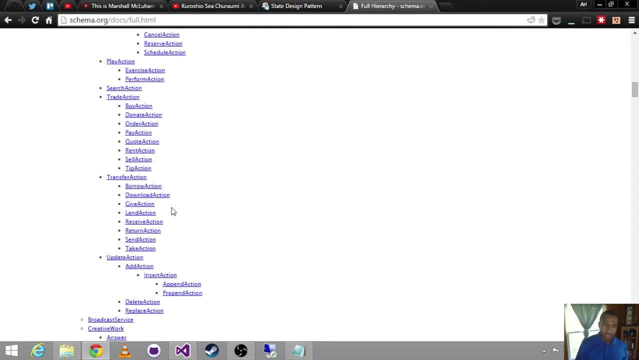 So it takes a thing and gives you a breakdown of what properties it could hold or should hold, And I've got quite a few Actions of different types: Answers, article blogs, clips, comments- And so modeling your business object can be half the problem. 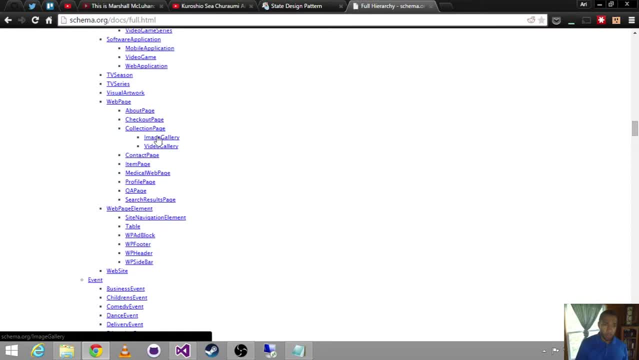 or half the challenge. So just pulling something and then I'll skip around. Yeah sure, Let's say you're doing a site that does job postings right. Again, data modeling is a dark field. It's a dark art in and of itself. 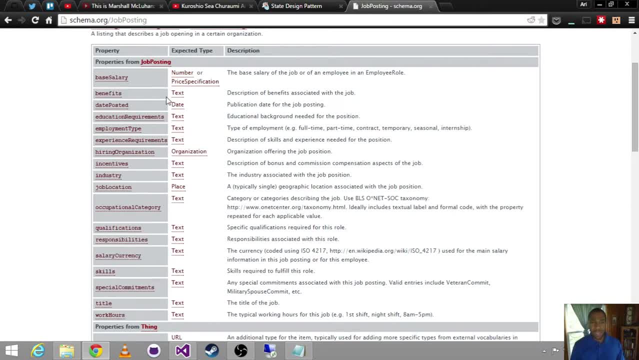 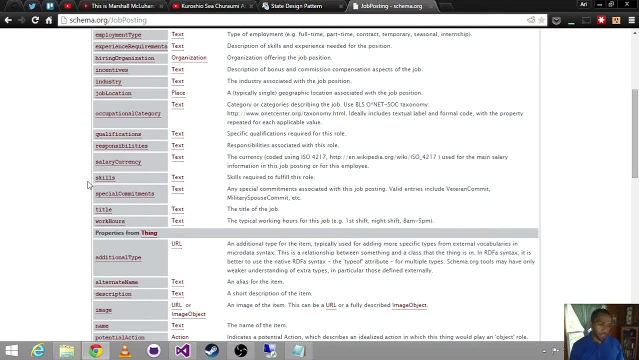 Maybe you need a kickstart on what that is all about. So here's some ideas. It's really nice in terms of I don't know what's supposed to be in this thing and or anything like this. before Give me some thoughts. 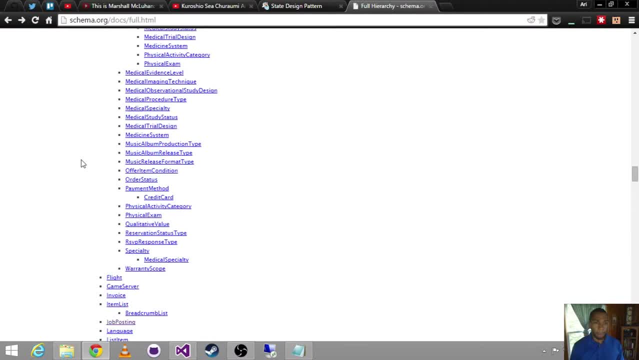 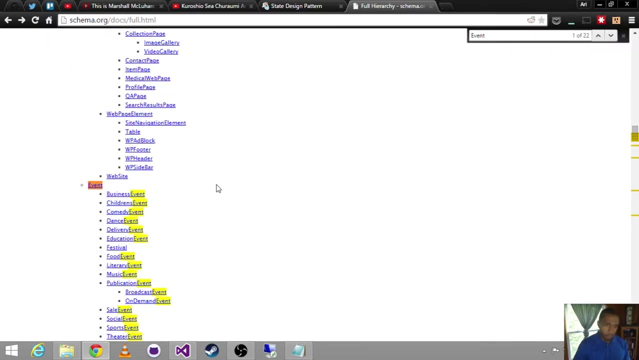 So I like it. I came here early and I thought doing an event would be good because we're doing the state pattern. So I'd make a really simple example And we're going to be doing very little of what they suggest. Let's say we had a social event. 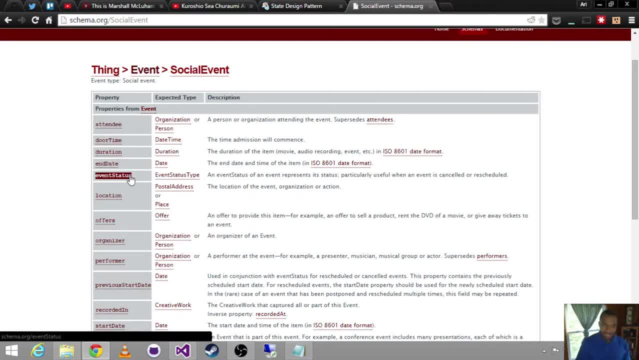 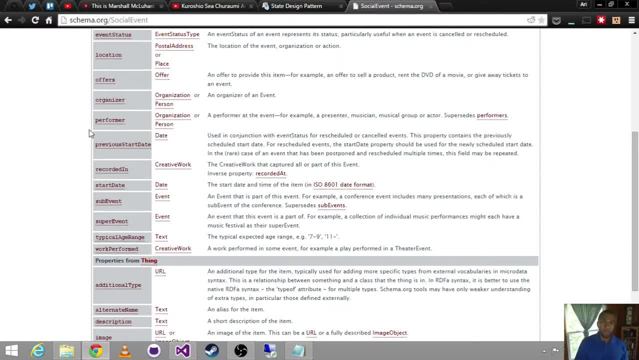 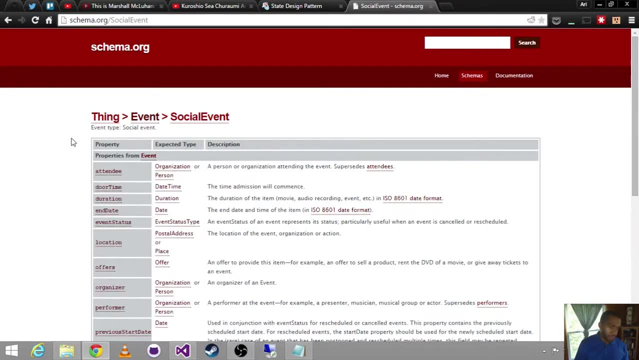 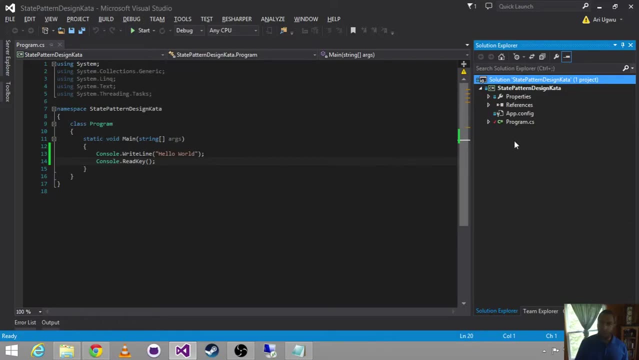 I think I could make a better event website or a better whatever. this is a great place to come and get some ideas for how you'd actually model that data. So under Arcata, we're going to go with an event of some kind. 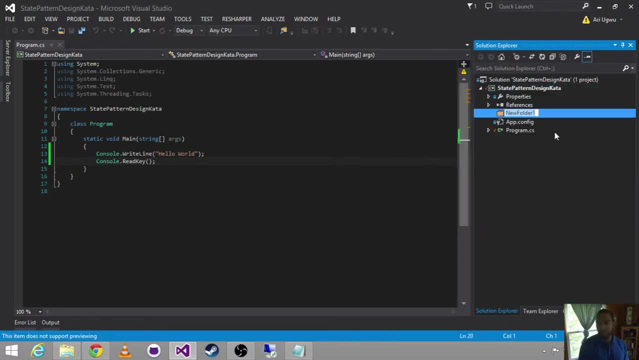 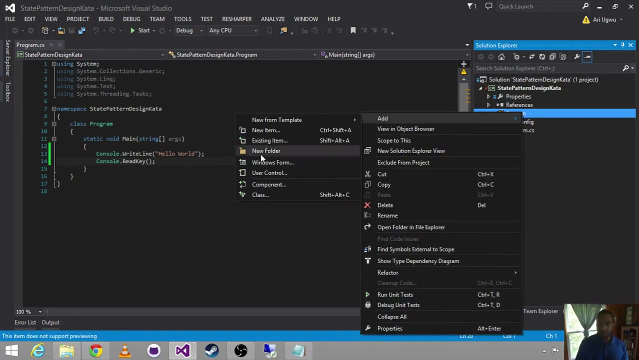 So let's go ahead and do a new folder and call that guy, get a new folder. And then let's say: OK, I'm going to do a section, a domain folder, super simple. I'm going to do a folder and we're going to say: social event. 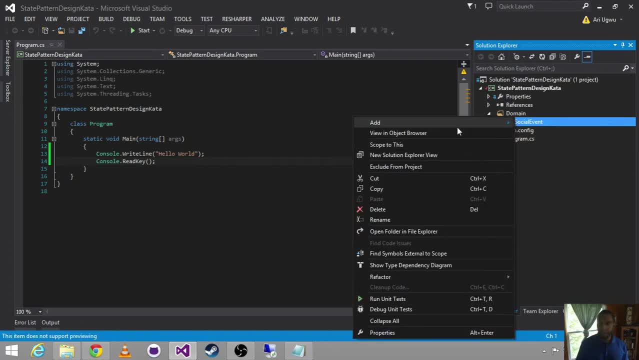 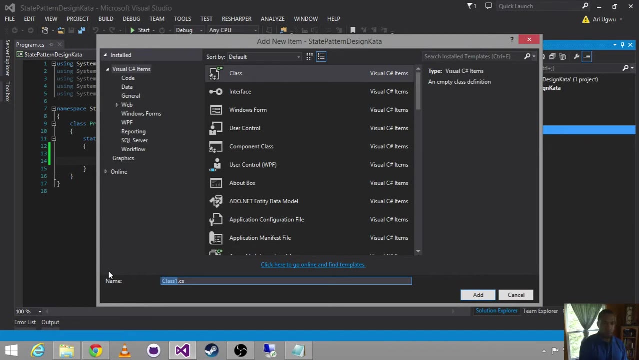 I'm going to do a new folder and we're going to say model, And then we're going to add a new class. Let's call it a social event. I'm going to put in my name and my name and what it does is we have a name. 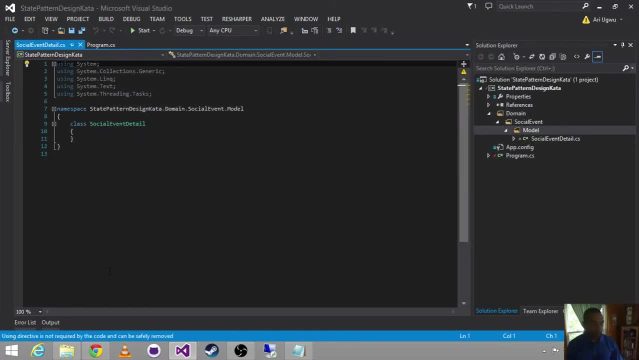 And how do I put my name in here? Let's call it the social event, All right, so let's just say that every social event is going to have a name as a property. I'm going to date time as a start time. 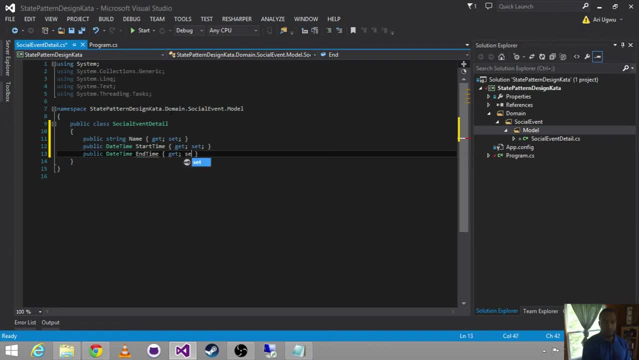 At name time, Pull this back up, okay. So we've got a domain name again. We've got the thing that we want to use to power our state pattern or be the target of our state pattern. So in the social event, and we're going to decide what state that event is in. 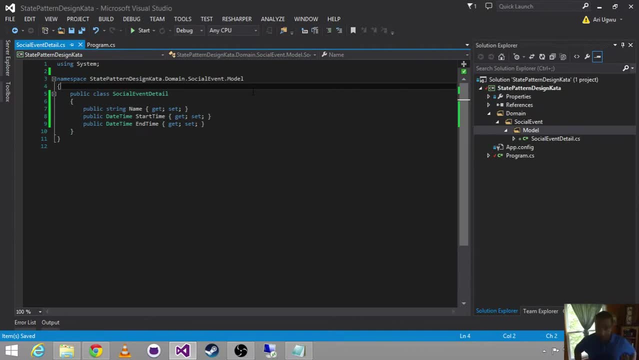 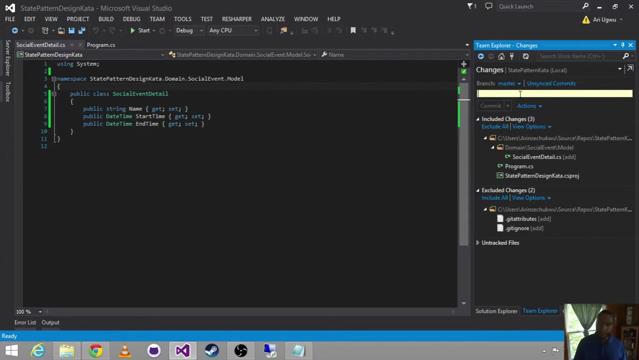 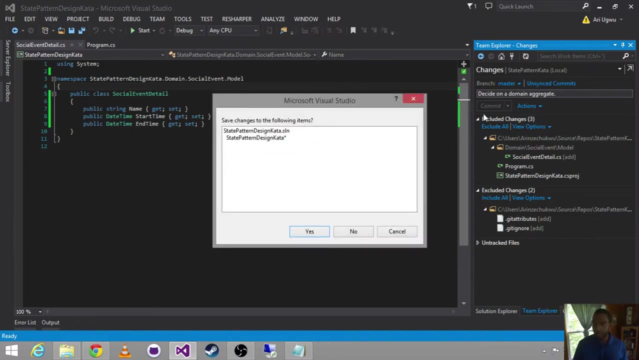 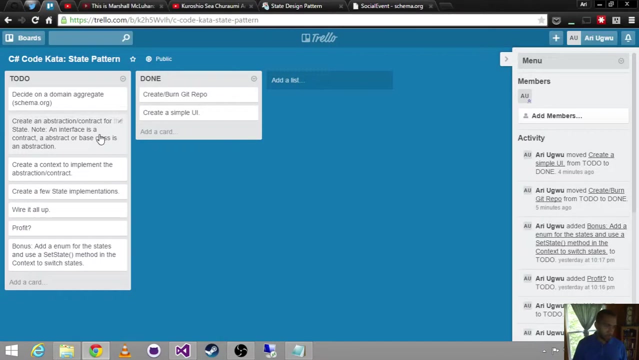 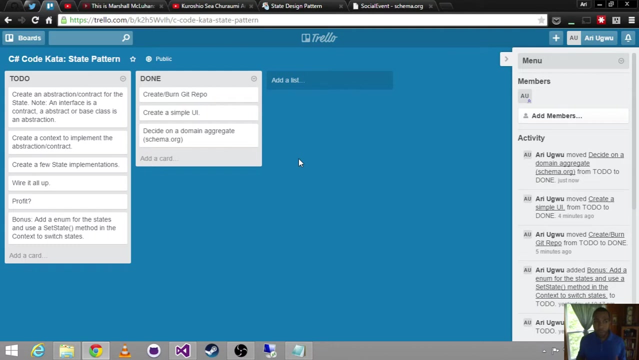 Is it upcoming? has it started? has it finished? So three simple states: I'm going to commit that, Decide on a domain. aggregate Commit. I will save And sync it. All right, so we're moving along, All right. so the next part of Mercado is to create an abstraction or contract for the 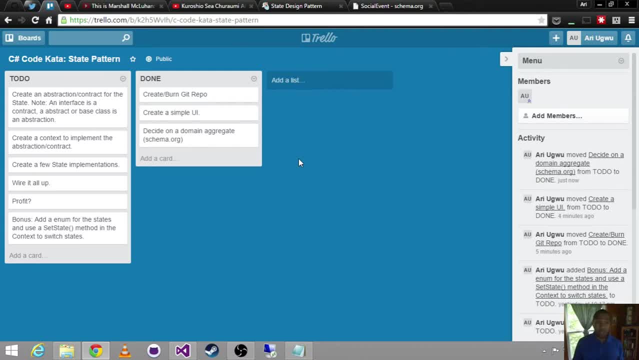 state, So a contract would just be an image. All right, so the next part of Mercado is to create an abstraction or contract for the state. That's an interface, And an abstract or base class is a true abstraction, Because we'll have things that any implementing classes need to implement. 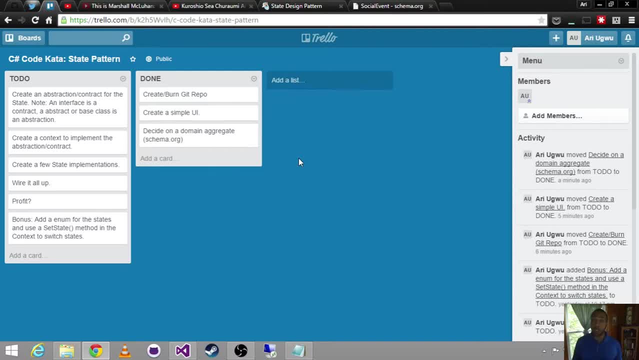 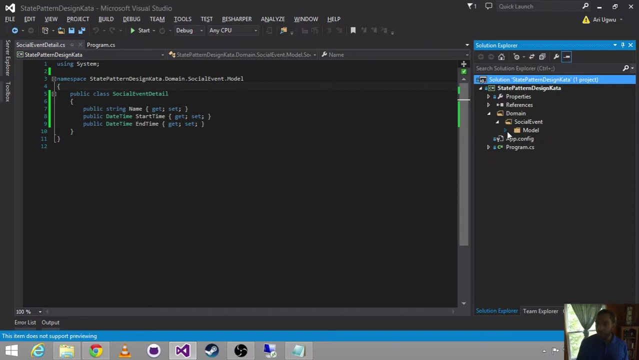 But we also are going to give some base functionality that ensures uniform behavior across the board. Okay, So, All right, So we'll come back over to our code. not inside a model, but inside our social event folder we can do a new item.